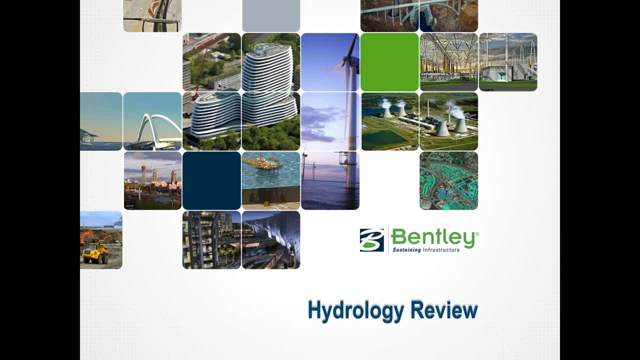 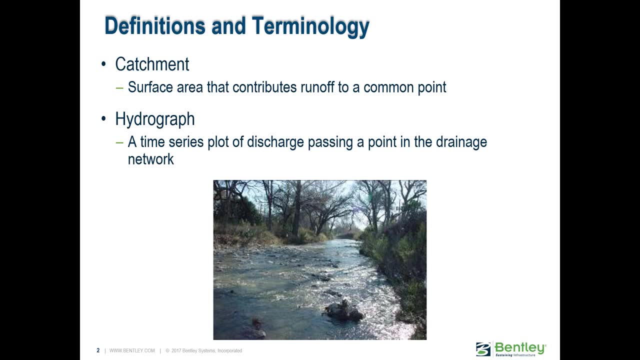 and figuring out what's the hydraulic grade line, energy grade line, velocities and things of that sort. All right, so the hydrology. the nice thing about this is that for StormCat the hydrology is actually quite simple: The basic definitions that we're going to need. 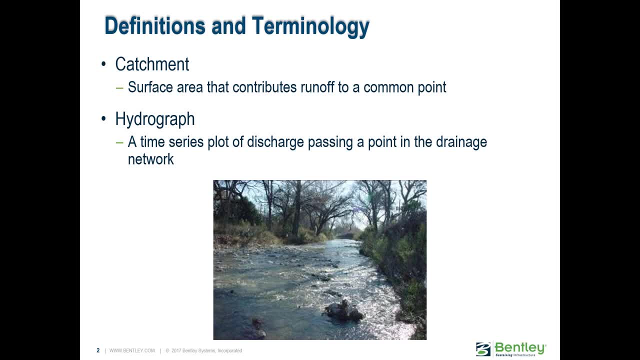 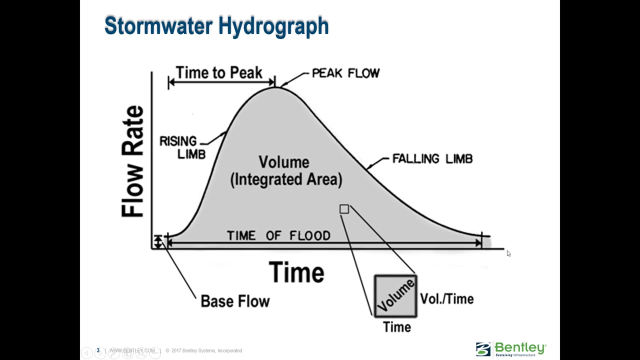 to know is: what is a catchment? A catchment is the surface area that contributes runoff to a common point, And a hydrograph is a time series plot of discharge passing a point in the drainage network like this. So basically we have flow on the y-axis and then time on. 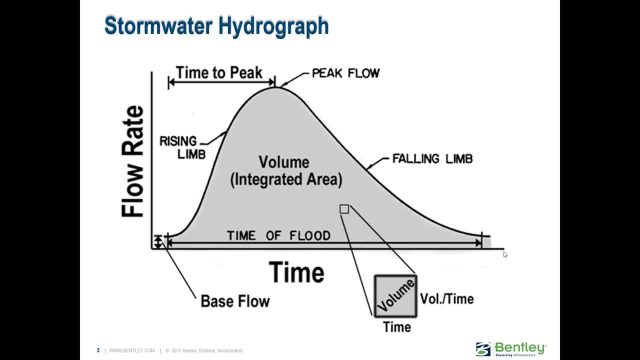 the x-axis. Now, remember that StormCat does only peak flow analysis, So when we're dealing with StormCat, we don't really need to know the entire curve. In fact, we're only looking at this one moment in time. We're looking at our worst conditions: peak flow, Okay. 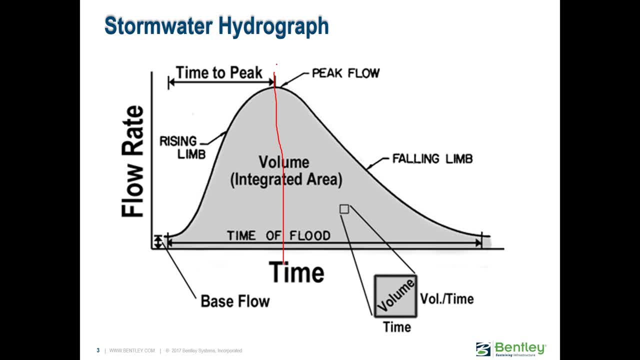 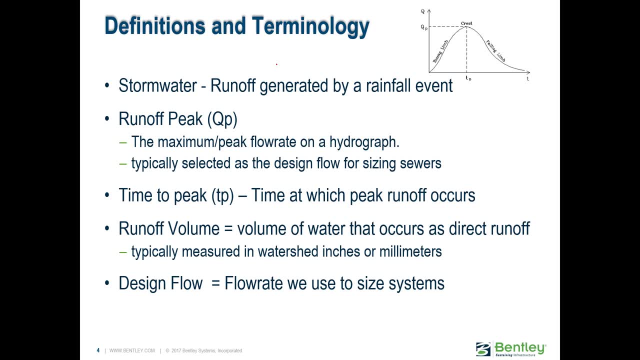 so we don't really need to know about the hydrograph and how things, how long it takes, No, we just look at peak flow, which is why the hydrology of this is so simple and great. Okay, So what we're concerned with is finding the peak runoff. so that value here And that. 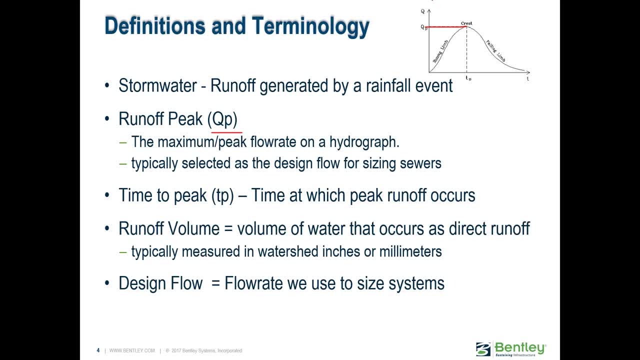 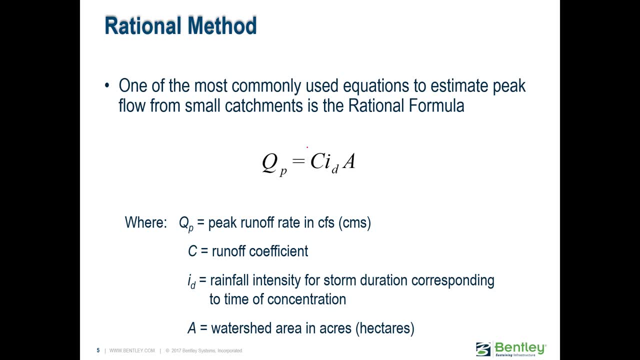 typically becomes the flow rate that we use to size our systems And, in the rational method, calculating that peak flow is the simple equation, which is the rational formula, which is C, which is the runoff coefficient times C. Okay, So what we're going to do is we're going to take the intensity times, the area, So for 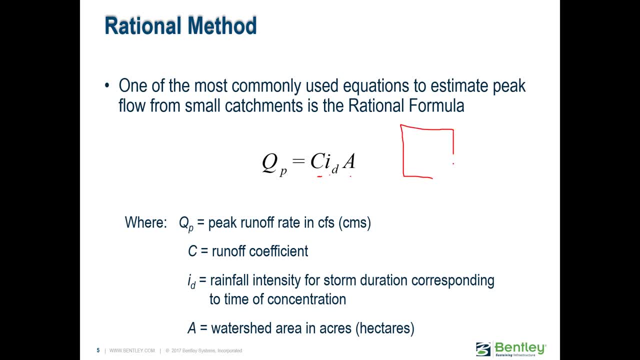 any given catchment. I'm going to draw a little square catchment here. We know it's area right. We know it's C runoff coefficient because we've looked it up in a table. So basically, if it's paved completely, the C is in the 0.95.. So it's like 90% of all the. 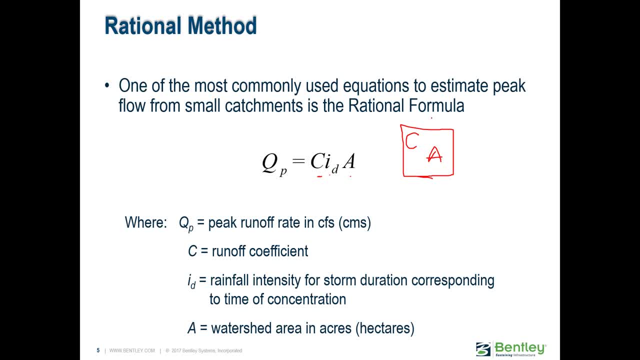 water. Okay, That would fall onto that square, will run off to its lowest point. Let's say it's going to be here. So if it's completely paved, you know it's like 90%, 95%, right, So that's. 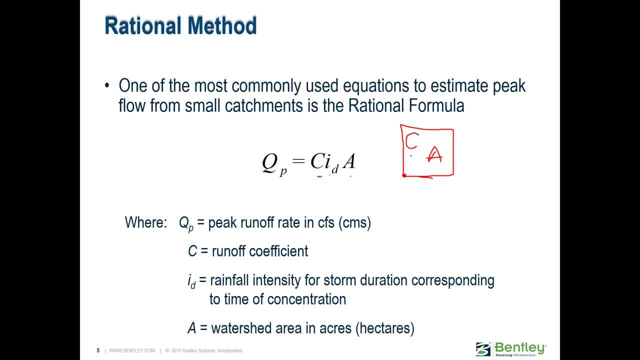 the C value. But if it's a very grassy area, we're going to be talking about C of 0.3, 0.4, 0.5. So like 30 to 50% of the rain that falls onto that catchment will become the 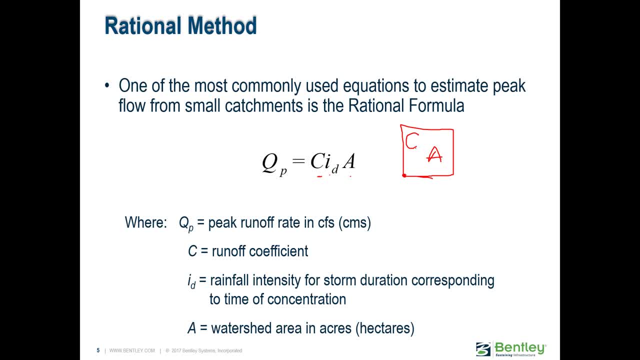 C. Okay, So that's really what that C value is. So where does that I value come from? The I is the rainfall intensity corresponding to the time of concentration. Okay, So we know that as soon as it starts raining, you know it's going to start raining everywhere in our square. 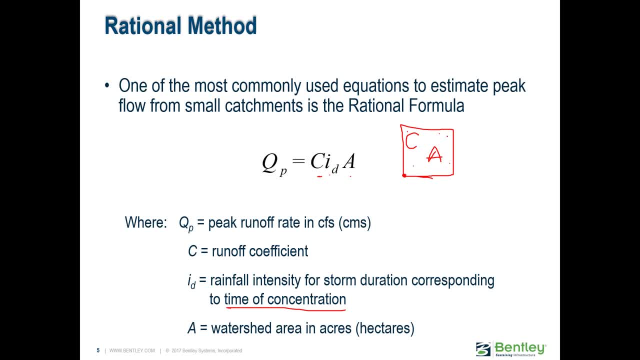 But the time of concentration is the time that it takes to a drop in the furthest point of our catchment to get from there to here. So that time is what we call our time of concentration Right Now. the intensity here is the intensity for that given time of concentration. Now let 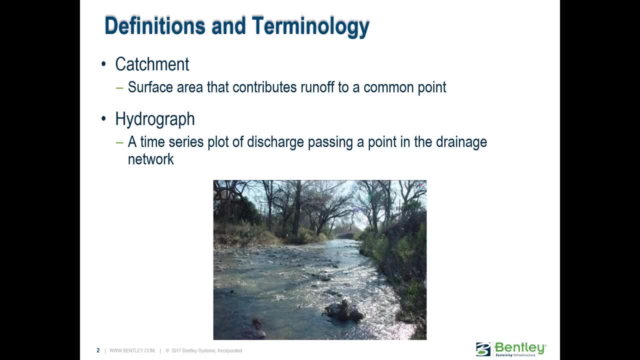 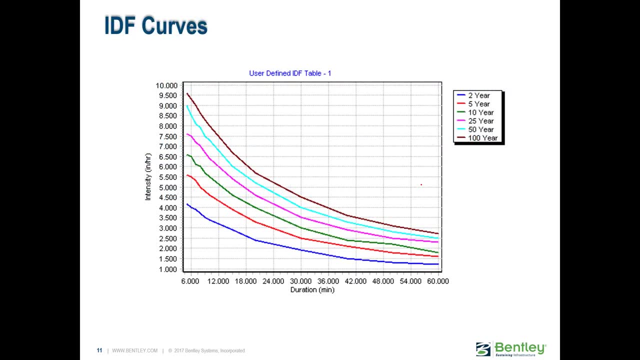 me back up a little bit and see if I can find my IDF curves. Where are my IDF curves Here? Oh, All, right, So this is what it looks like, Okay, Okay, So this is what an IDF curve looks like, Right? So it tells you the intensity in inches per. 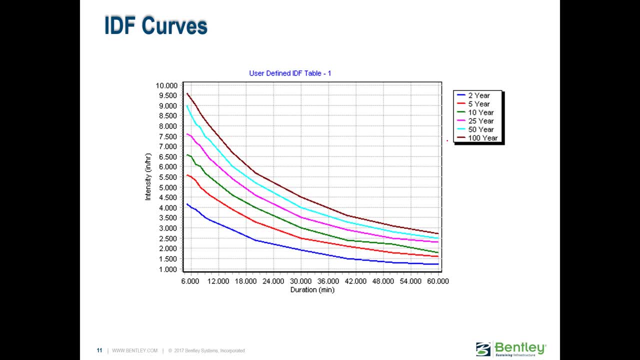 hour for different return periods, So two year, five year, ten year, etc. So let's focus for the two years. So we say in our square catchment there we figured out the time of concentration was however long it took that drop to get from that corner to the outfall. 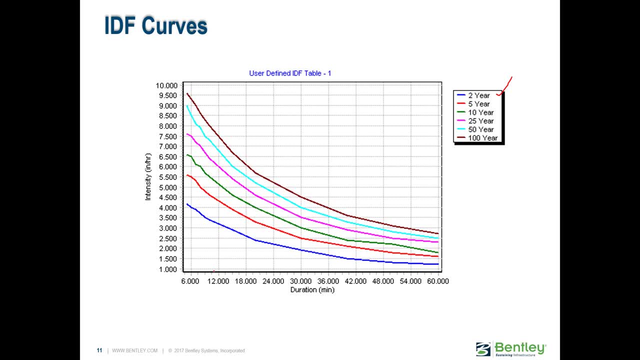 Let's say it was 10 minutes to make it easier. And let's say 10 minutes is here. So if my time of concentration was 10, then the intensity that it will use to calculate that Q equals CIA. this is the I I would be in this case. 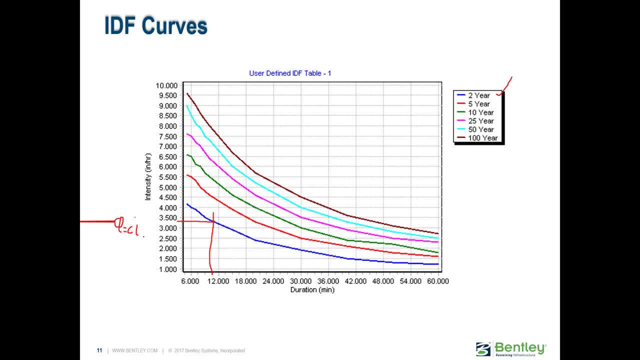 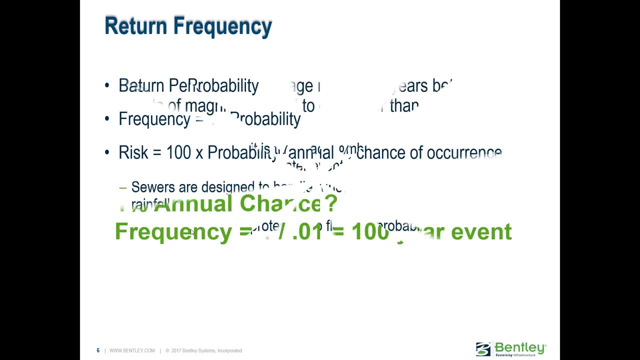 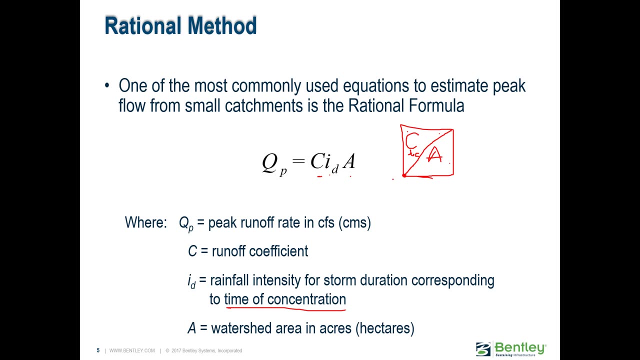 3.3 inches per hour. So let's go back. So here's our. I Correct: This is how simple it is, guys. It really is that simple, All right. So we looked at that time of concentration, looked it up, basically on that duration part. 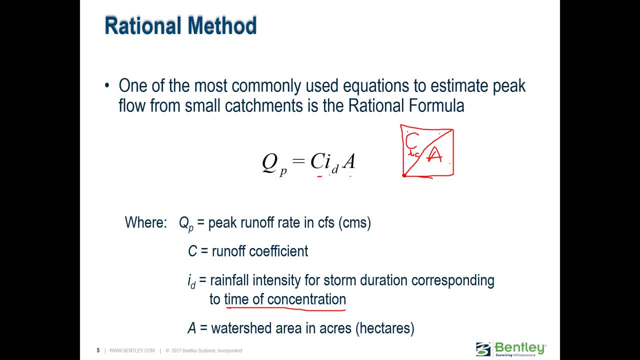 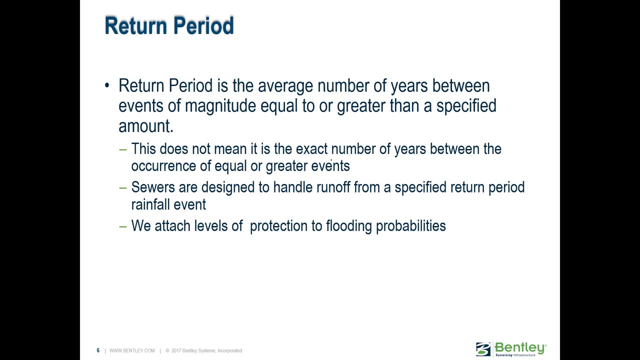 of our IDF curve figured out, the- I multiplied it here- times CIA, and that's how we got our peak flow Very simple, right? Okay, But our peak flow is different for each of those return periods, right? So I did the example for a two-year storm, but obviously the duration, the IDF curve for a 100-year. 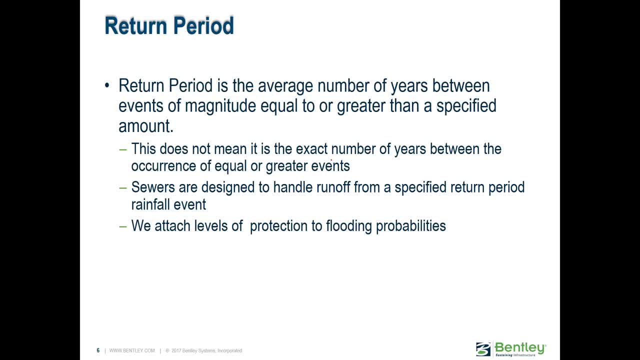 storm is going to be different, So we basically have peak flows for each return period. Okay, And what is a return period? It's the average number of years between the events, of magnitude equal to or greater than a specified amount. This is a mouthful to say that this is probability. 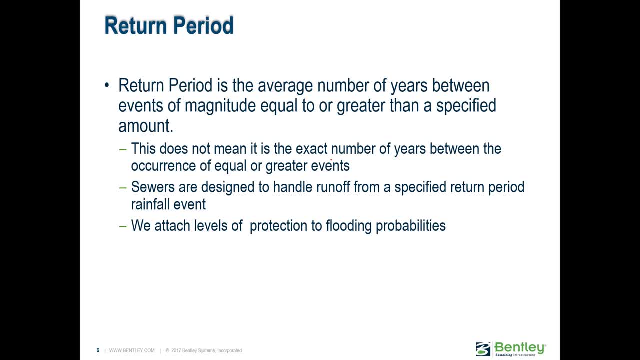 So we looked at how much it has rained in the last X number of years. The more data the better. And then we make predictions. We say, okay, well, the probability of having a storm of this, you know 5 inches depth or 10 inches depth, or for each of the depths we figure out what is the likelihood that. 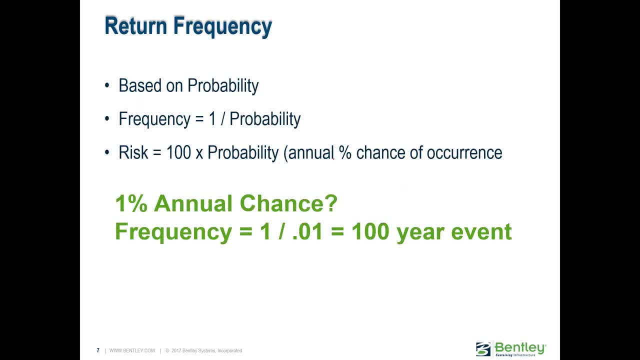 that would happen. And again, it's based purely on probability, looking at historical data, And then we say that the storm frequency is the inverse of the probability that that event is going to occur where you are during those IDF curves. So, for example, if there is a storm that has a 20% chance of occurring, 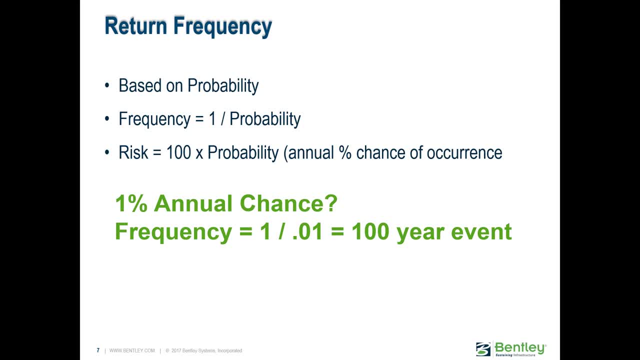 your probability would be 0.2.. So what would be the frequency? So frequency would be 1 divided by 0.2, and that gives you 0.2.. Number five, five, what Five-year event. So that's how we defined our two-year, our five-year, our 100-year: storms. 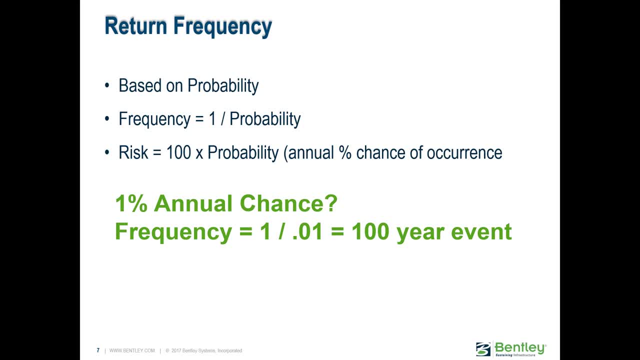 So the most probable storms are going to be- you know so, like a storm that has a 90% chance of occurring- would be 1 divided by 0.9.. So it would be a smaller number, right? So that would probably- I don't know my math right now- 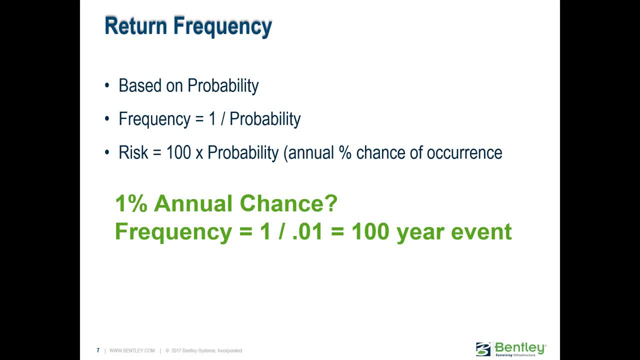 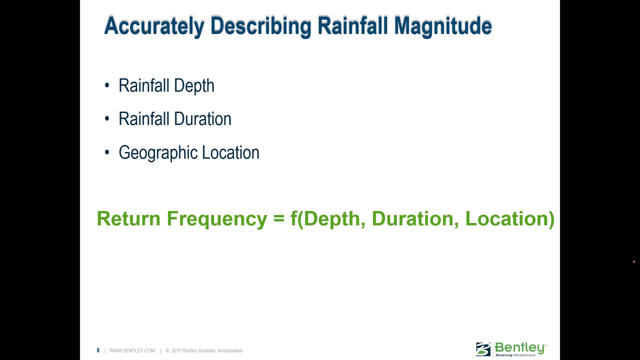 but my math, but it's probably going to be a one-year storm or something like that, Right, Because it is very likely to happen at least once a year. So how do we define our storms? Well, we decide what is the depth, the duration and where you are located. 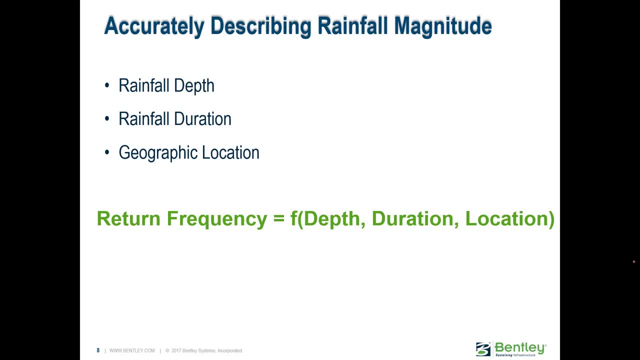 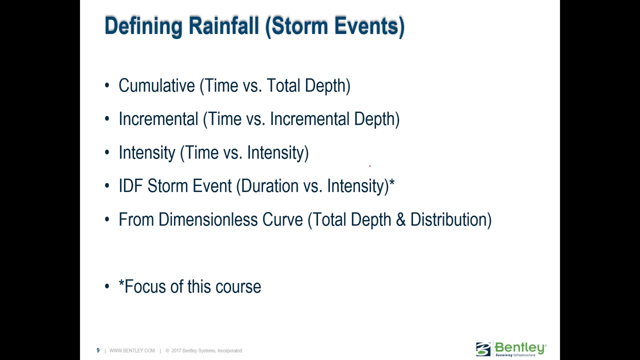 Yeah, so it's not the same to have an IDF curve for Columbia, where I am, as it is for Denver or anywhere else. It's unique to your geographic location. So there are different ways of defining storm events. You can do cumulative so you can just basically figure out how much, how many inches of rain you got every single day. 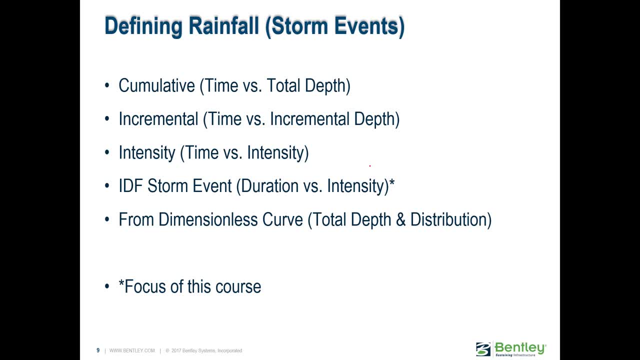 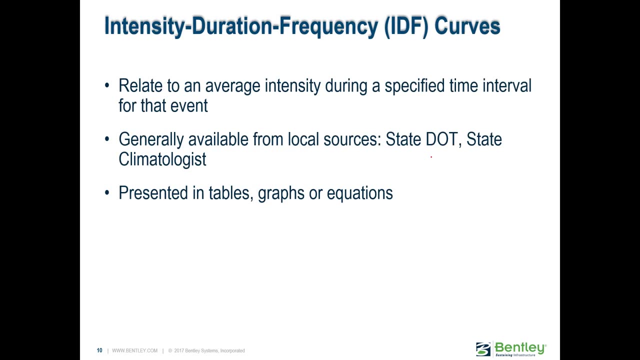 for a whole year and things like that- incremental, But for ours we basically use those curves based on the historical records at our location and we define intensity, duration and frequency for each of our storm events. So again, this is a way to simplify our storm events that are happening in our area. 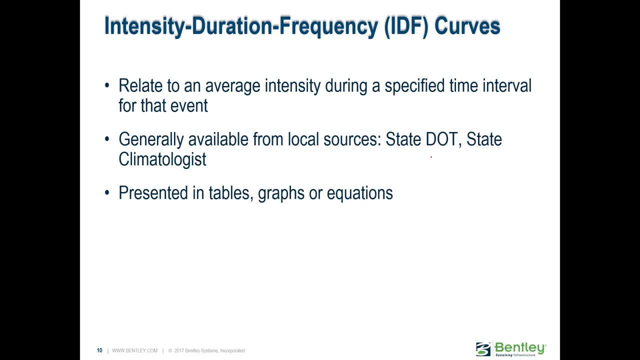 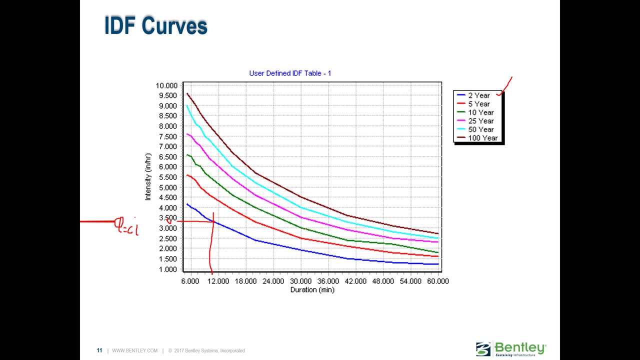 Typically, you get this from your DOT, the state climatologist, and they can give it to you in a table or a graph, or simply give you some equations, But ultimately, what they look like is like this. So it's a family of curves that you see here, each of the curves representing a different frequency. 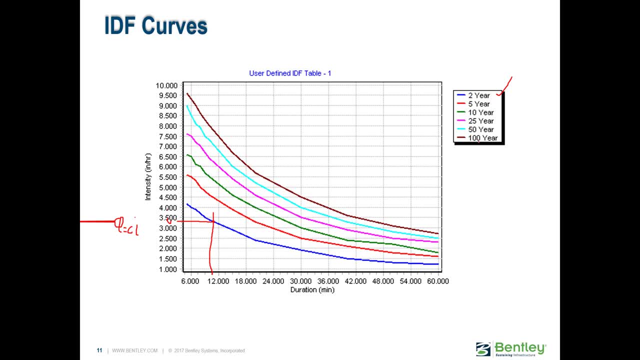 So two year, five, up to 100 year in this case, And basically just tells you what is the probability of you having a 24-minute duration storm in any given frequency and what would that intensity be. So it's our way to project into the future. 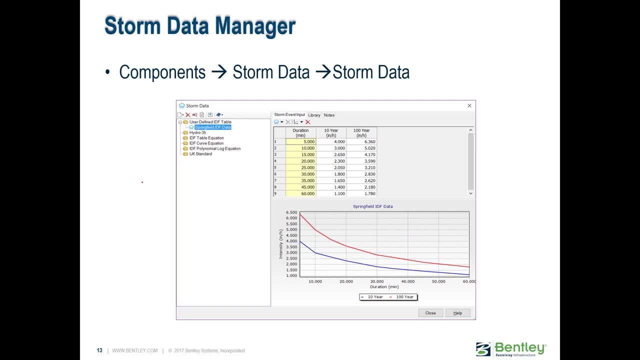 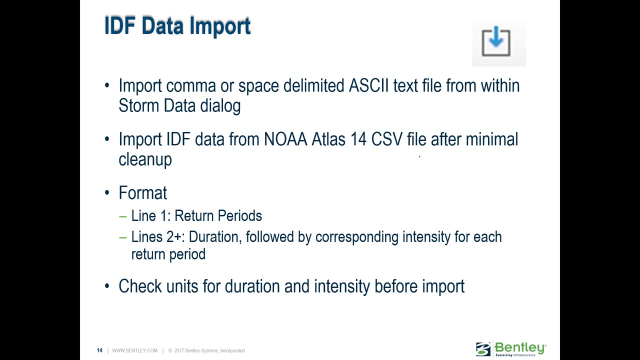 All right. so you went to the DOT or your state climatologist and you got your IDF curves. You open StormCat and you go to components- storm data- and you input your IDF curves. You can import them from text files directly or you can copy paste from Excel. 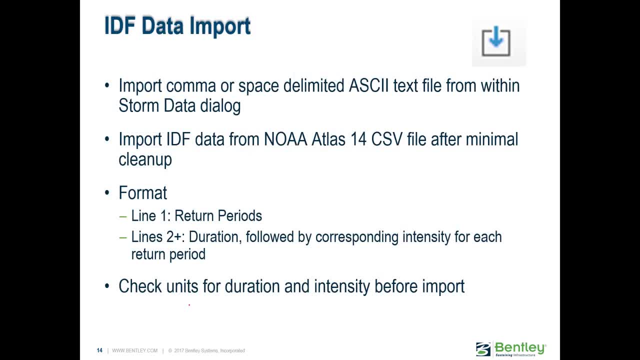 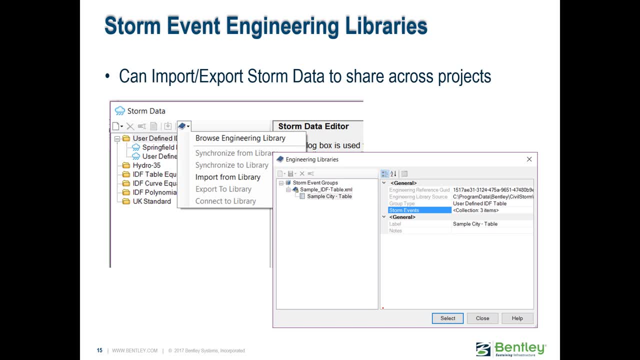 Important here is: make sure that you are checking the units for whatever you're importing, So for your duration and intensity, And if you're going to be working in that particular area and you're going to be reusing that storm data a lot, then export that. 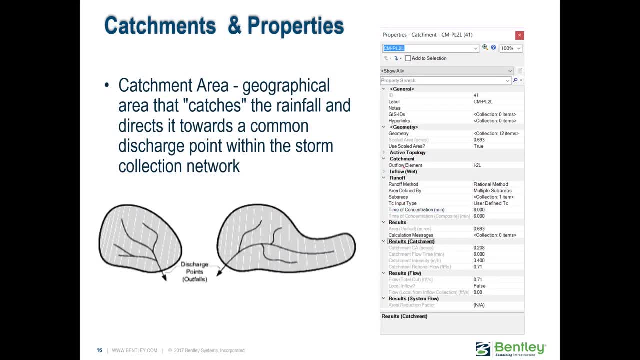 Enter it once and then export it to your library so you can use it for all your projects. All right, so now we know where we get our storm data, what it means, those IDF curves, And what do we do with that? We put it in StormCat. 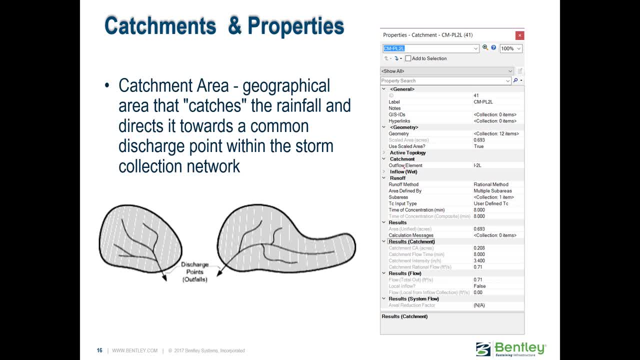 Now, what else does StormCat need to figure out the hydrology? Well, it needs to know all about that catchment. So here's a little screenshot of the properties of a catchment. So, basically, you specify how you want to define the area. 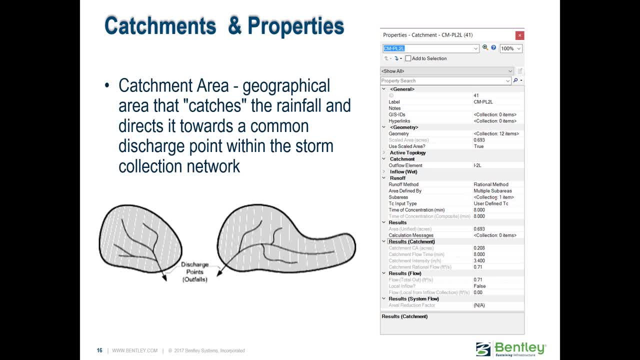 You could have sub areas or you could have it all be one kind of an area. So if you have a catchment where parts of it are paved but the other part is grassy or different sea coefficients within that catchment, then you can use those sub areas. 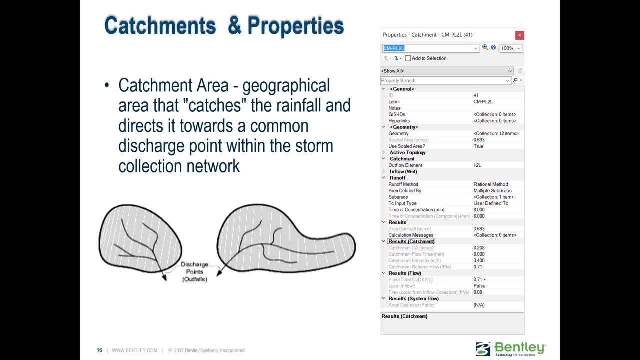 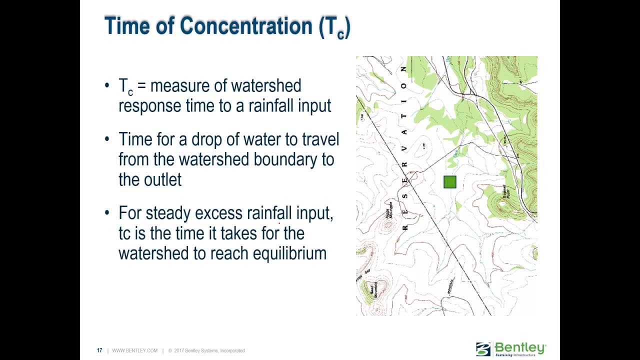 So you need to input that and you need to tell us the time of concentration And in fact, in the software there are 13 different methods available for you to come up with that if you don't know it already. As we mentioned, the time of concentration is the. 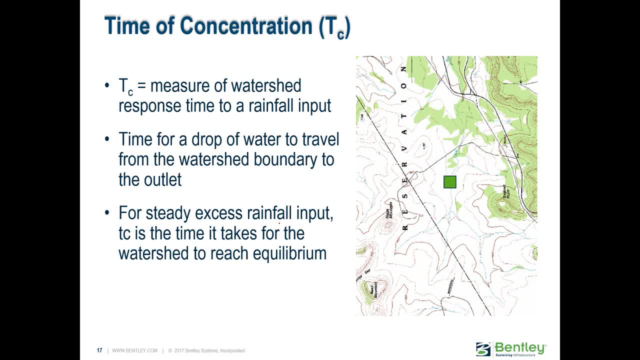 time. it takes a drop of water to travel from the watershed boundary to the outlet. So here's our boundary and the longest path, And we take a look at all the paths, figure out which is the longest and time it. So how do we do that? 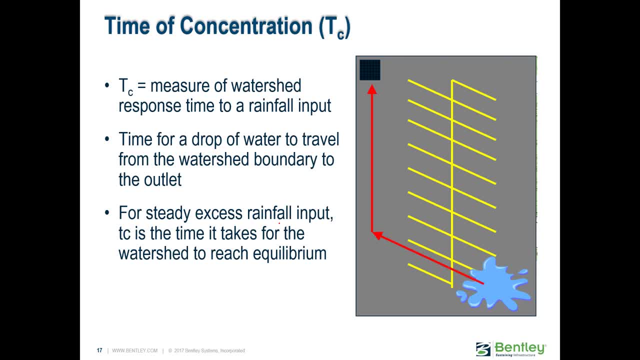 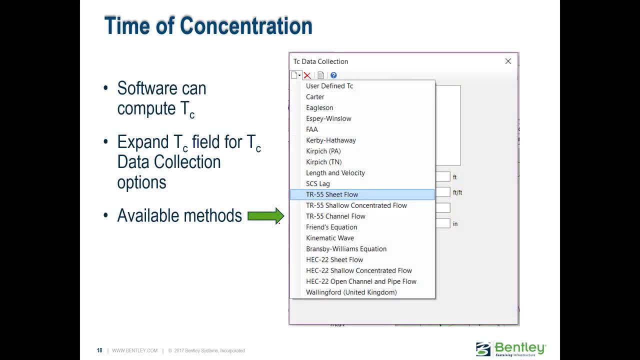 Here's again an example of the drop of water traveling in that direction. There are different methods. If you've already calculated it somehow, you can simply enter that value, or you can use any of these equations that are found here. Most of the equations will tell you what is the actual length and what's the slope. 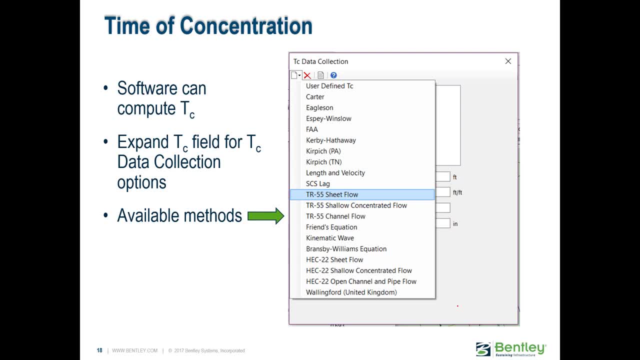 That's the minimum. Others would say: what's the length, what's the slope and what kind of surface is it, so that I know if it runs really fast or if it's like a bumpy road where that drop is going to take forever to get there? 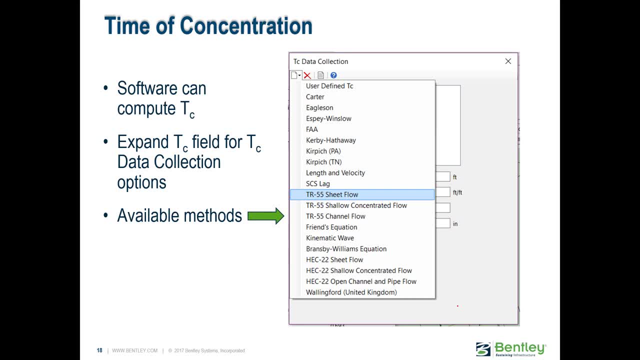 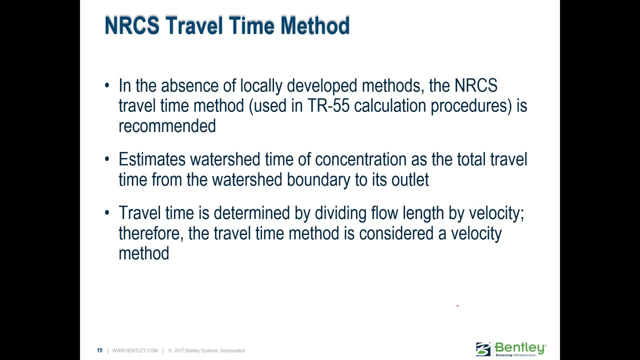 So, in a nutshell, that's what you need to input for time of concentration. Okay, so if you don't know what you have to use, if nobody's defined what methodologies you're going to use, we recommend that you use the TR55 methods. 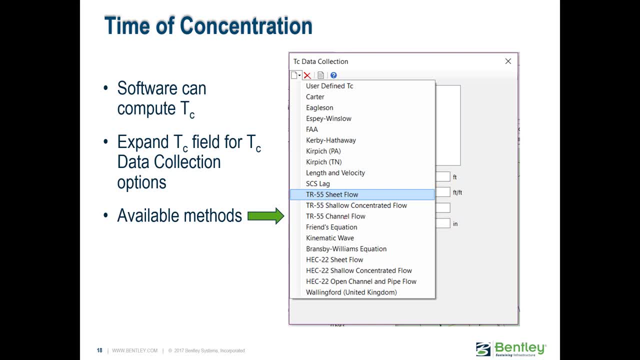 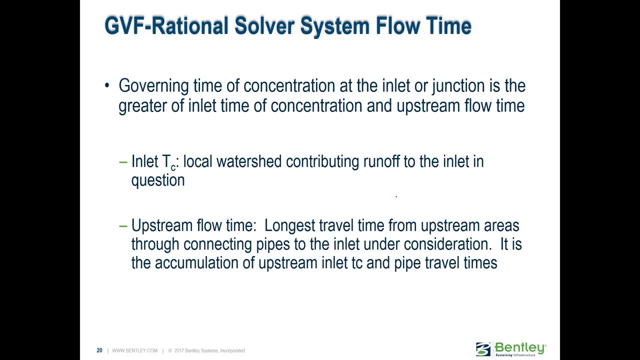 You can see here the sheet flow: shallow concentrated flow or channel flow. Okay, so you're going to notice, as we do more of these exercises, that there is something that StormCat uses which is called the system flow time, So it is easy to see the time of concentration on a per catchment. 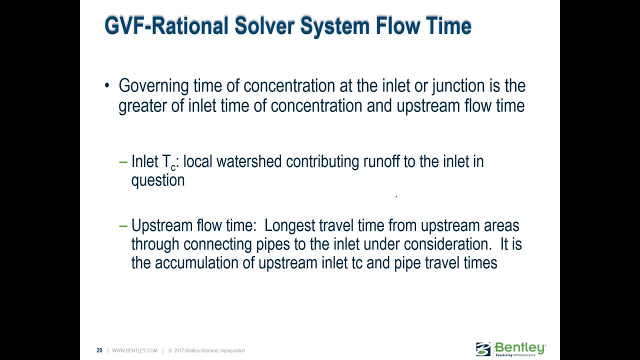 on a per catchment basis, right. But most of the time your model is not just going to be one catchment, It's going to be a series of catchments. So it rains, the runoff from that catchment goes into the storm system. 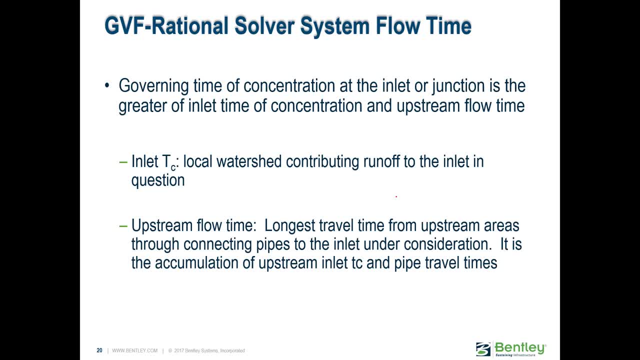 you know, into your pipes And then from another catchment you are getting flows. So we need to figure out what is that system flow time? And basically what that means is that it's the governing time of concentration and we look at the time that it has taken for the flow to arrive from an upstream inlet. 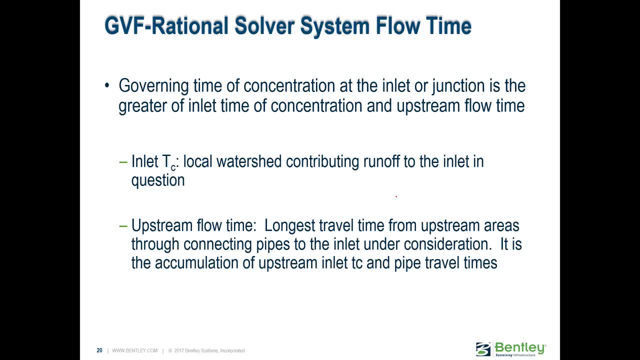 which is what we call the upstream flow time, and we look at the time of concentration at that particular inlet where you are. It's basically we look at which is greater of those and that's what we use as the system flow time. And why am I making a big deal about this? 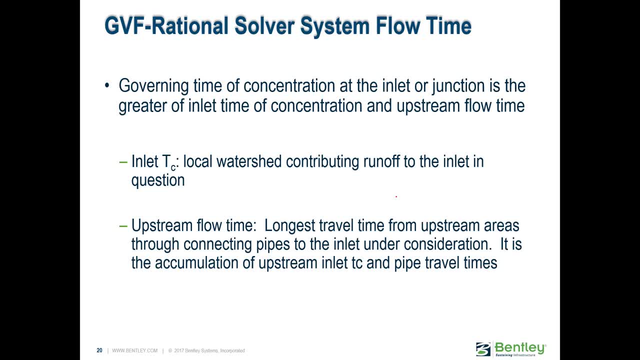 You know, it's something that the software handles on its own. Well, that has an implication that you might encounter at some point, and is that it seems as if there were flow discontinuity. So you say: okay, from my most upstream catchment. 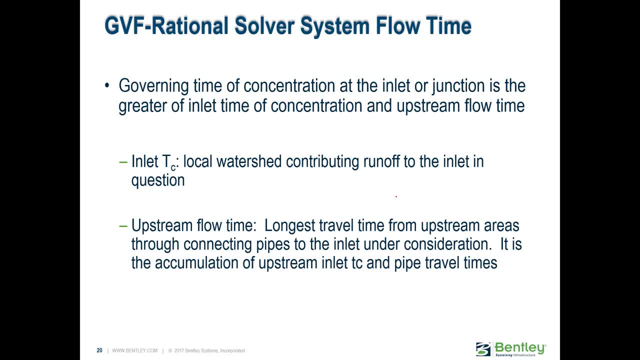 you know I got X number of flows, X number of flow units. you know I hesitate to say gallons per minute or liters per day or something like that. Let's call it flow units. So you get X flow units from your very first catchment. 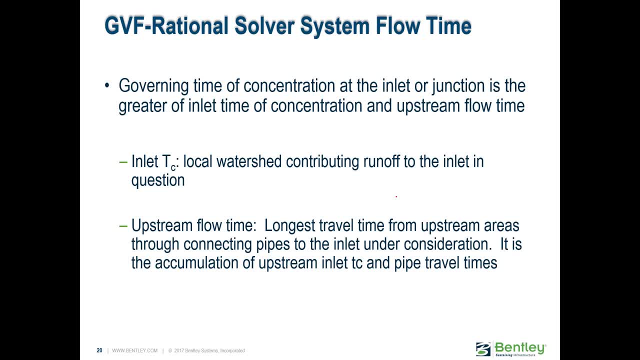 and then that flows down the stream And then at the next junction it makes that calculation of, okay, what is greater, the time that this flow has been in the system versus the time from this particular unique catchment, and it might be that it recalculates your Q, your peak flow. 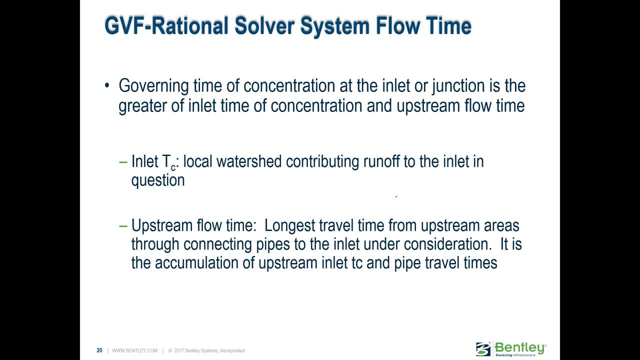 So your peak flow is no longer the X that you brought from your upstream node. It turns out that it's less. And then you think: well, what happened to my flow? It's no longer X, but it's, let's say, 1.2X or 0.8X. 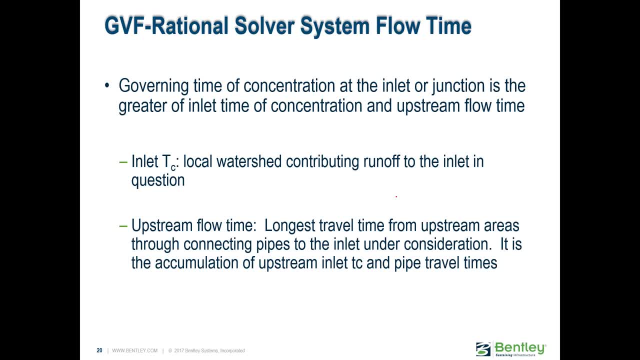 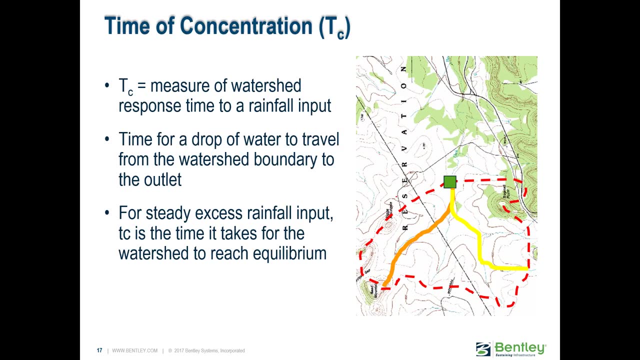 It sometimes shows as flow discontinuity. but it's not flow discontinuity. It's that if we, the longer the time of concentration, the less intensity, right, Remember those IDF curves. Let me go back here for a minute because this is important. 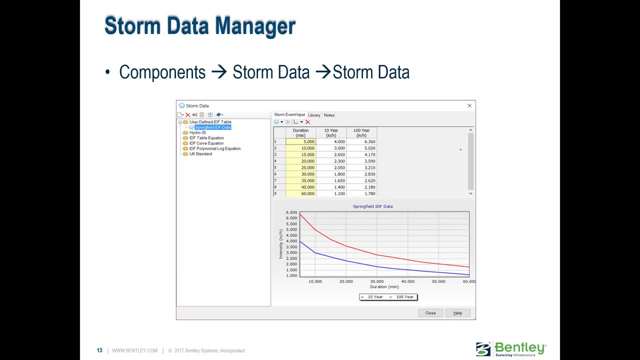 It has happened to me so many times that people get confused that I feel like I need to spend the time to really explain this. well, So this is our duration right. So the longer the duration, the less intensity. therefore, the less peak flows, right. 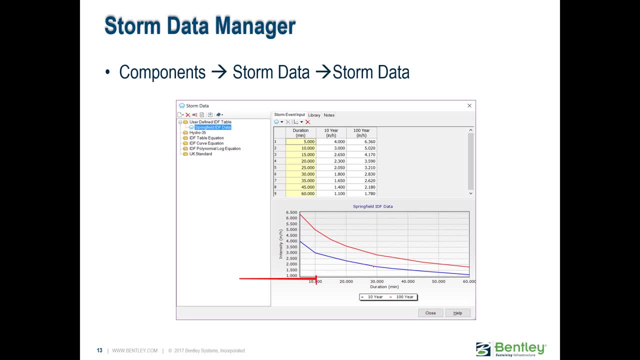 So if the time of concentration for your system has extended to be so long that the peak flow is assumed to be- let's say this was going to be our intensity, so your peak flow is going to be a lot less than if the time of concentration had been only 20 minutes. 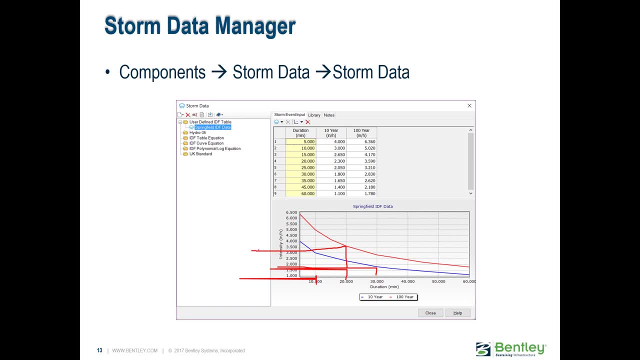 where your intensity would have been this right. So that is the implication. So some people would say, well, it's more conservative to always use the shortest time of concentration, but then you're actually going to end up oversizing your pipes as well, right, 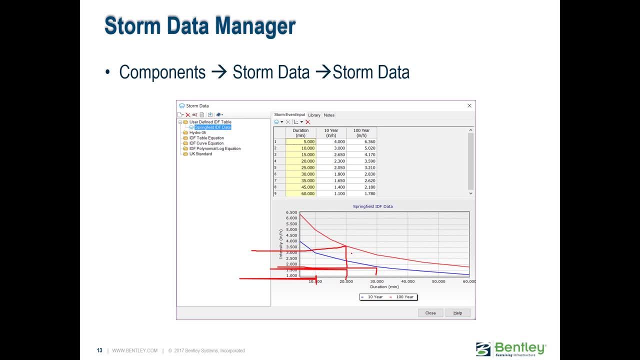 Because you're assuming a peak flow. that's never going to happen. And why do I say that it's never going to happen? Because flow does attenuate in your pipes, you know. So if the peak flow occurs- you know a mile from where I am. 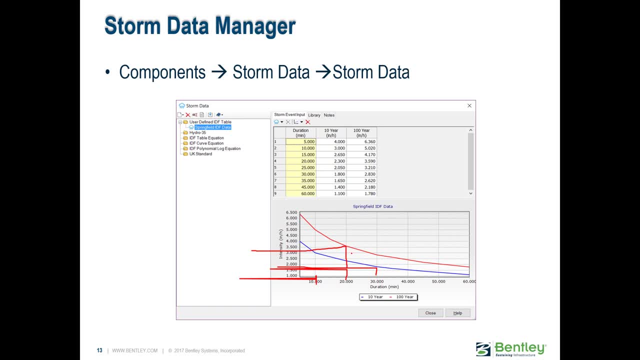 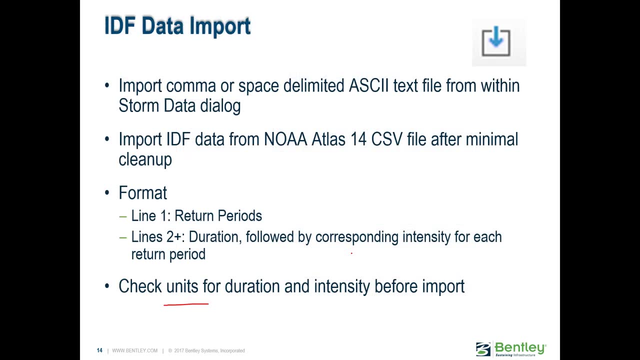 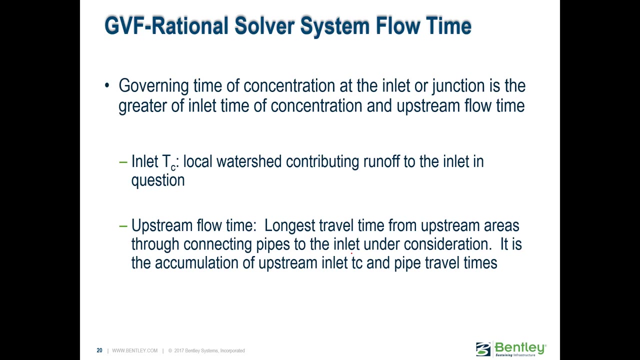 you know it happens instantaneously, but by the time it gets here it has reduced dramatically. So that is why we make that recomputation at each node for that system flow time. okay. So because we don't want to way overestimate. 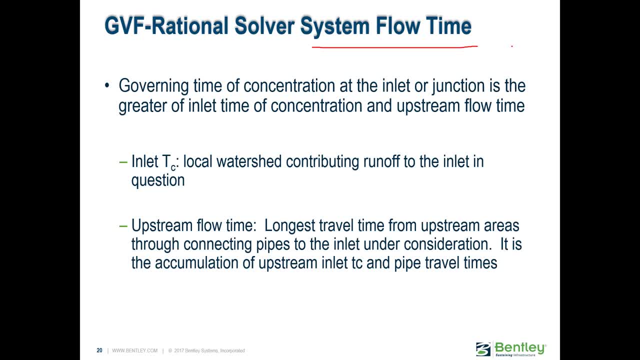 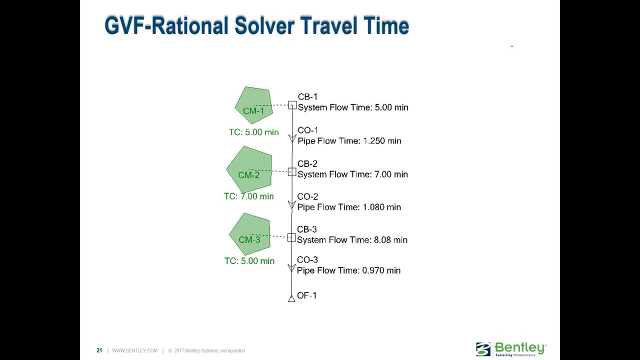 the peak flows, you know, because there's attenuation between the time they occur and the time they get to you. Alright, so here's an example of what I just explained. You have all different catchments, So you have three different catchments. 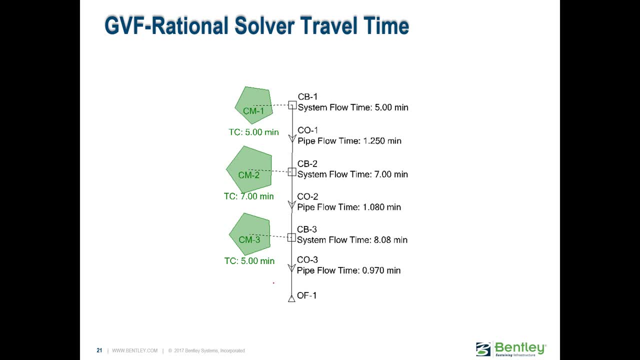 and each of them has a time of concentration. You're going to see that at the very first catch basin the system flow time is 5 minutes because that is the time of concentration for your first catchment. Then you know that it takes 1.25 minutes. 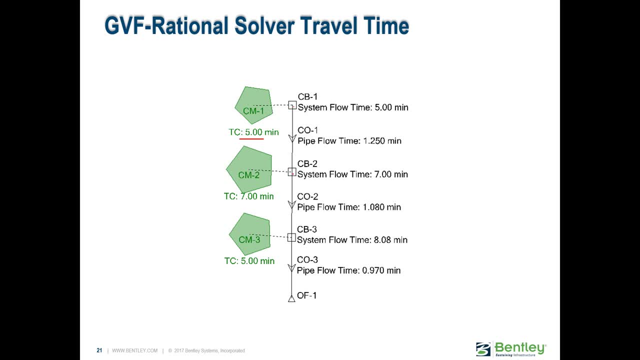 to get from CB1 to CB2.. So you would say, okay, the next system flow time it's 6.25.. But no, it is actually 7 because, like I said, it looks at every single one of your nodes. 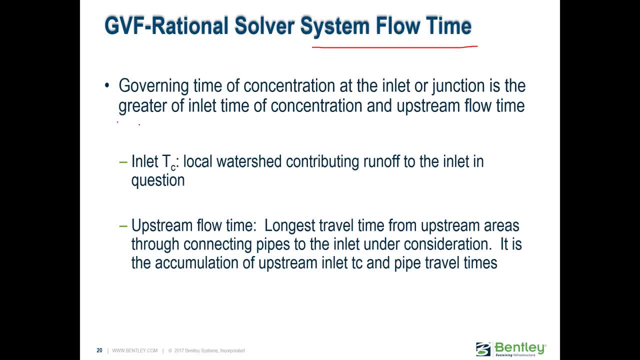 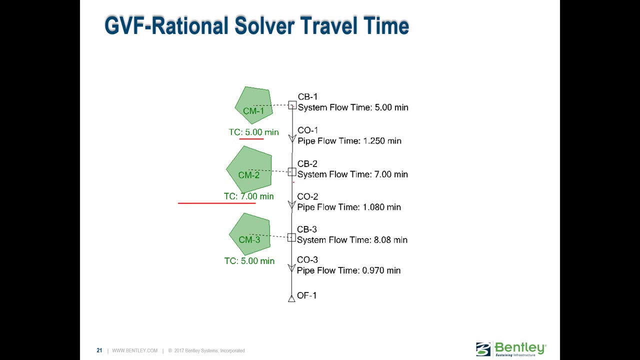 and it looks at which is greater: the time of concentration in that particular inlet or the upstream flow time. So it says ah 7 is greater than 6.25.. So my new system flow time is going to be 7.. 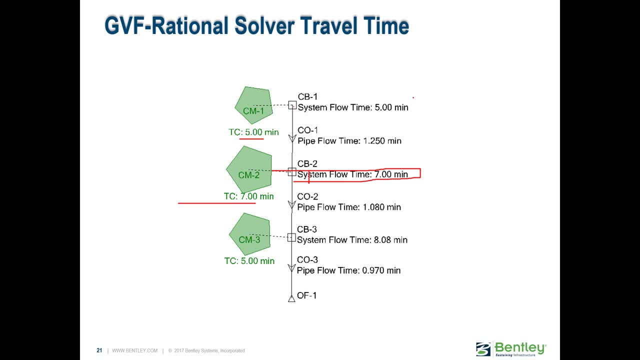 Now the flow that would be calculated would have. that's where I'd say you might see flow discontinuity because of this. So it's not like the flow is going nowhere, It's that we're just using the greater of the times between the time of concentration. 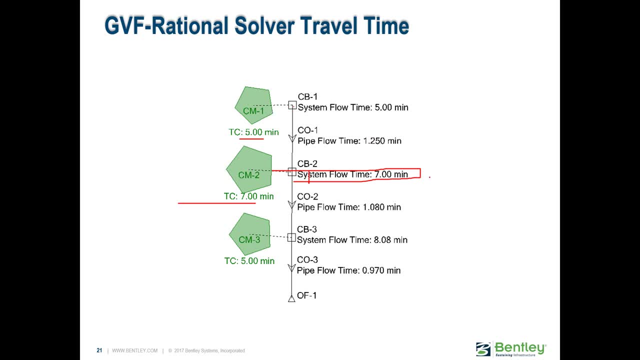 and the travel time to recalculate our system flow time. Now let's keep going down here. So 7 minutes plus 1.08, system flow time 8.08 versus time of concentration of 5 minutes. So we always go with the greater. 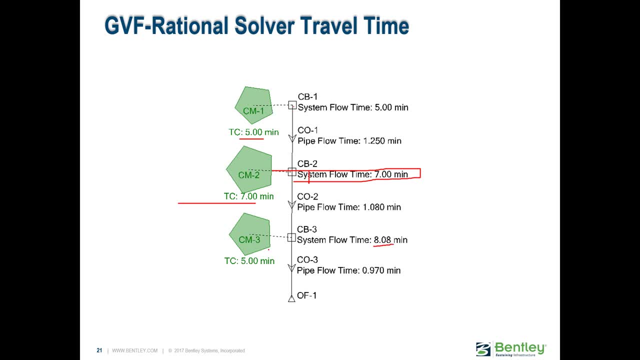 So 8.08 is greater than 5, so we're going to stick with that, And so by the time you get here, the new system flow time would be 8.08 plus 0.97.. All right, so don't worry. 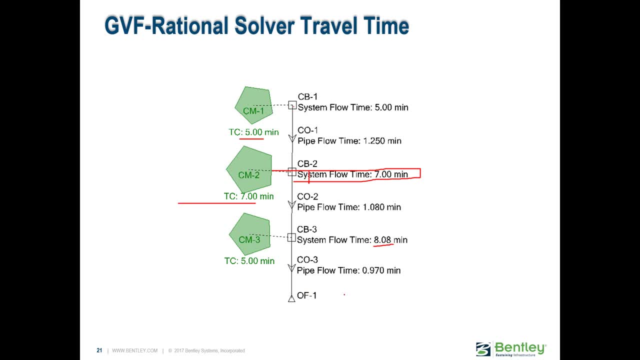 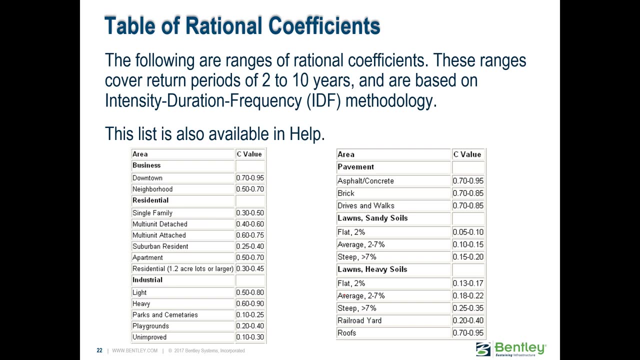 if this doesn't make a whole lot of sense right now, When we're doing the equations, you will see exactly what it is we're talking about. Okay, so we said again: our equation is: Q equals CIA and the C is read from our traditional tables. 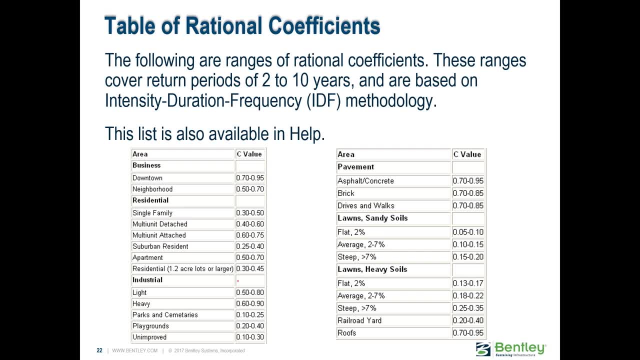 So you just Google it if you don't have it, and you'll be able to find these tables that tell you that, depending on the um use of the soil or the pavement or the the, how permeable your soils are. 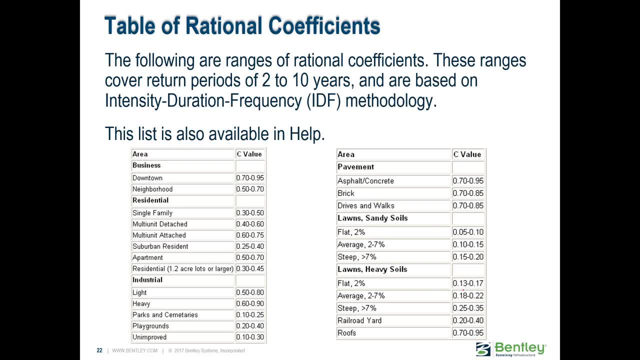 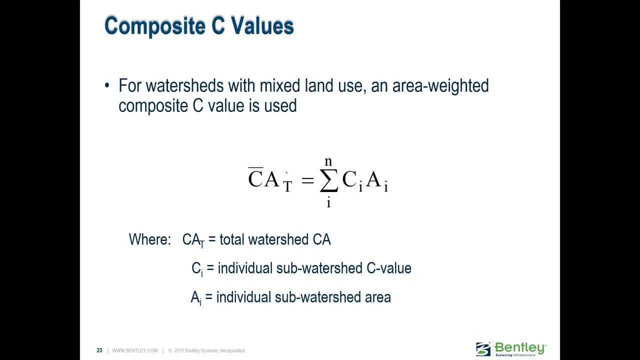 your C values will be different, So you can have anywhere from 0.13 to 0.99 in theory. Okay, so I said you could have a catchment. that is, you know, some part of it is a. it's a grassy area. 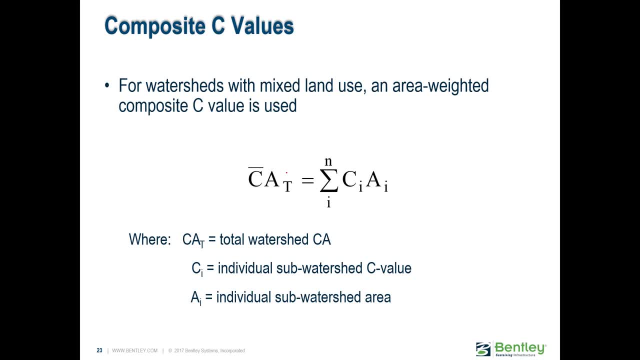 another part is a paved area, some roofs and things like that. You could have all of them represented as one catchment, but then you'd have those um sub-areas and each of those would have its own C value and then the software would take care.